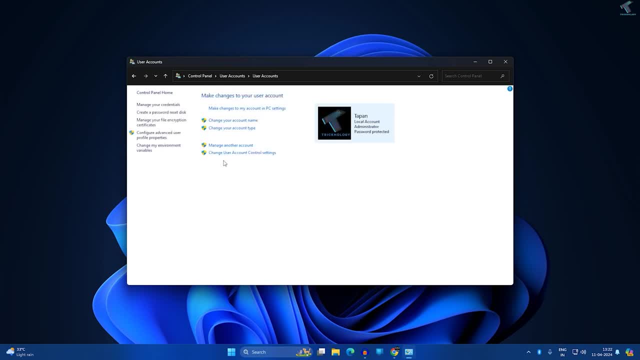 now go to user account once again, and here you will get option called change user account control settings. now you just need to click on that option. now here you just need to select neighbor, notify okay and after that click on okay. once it will done, you just need to restart your pc. 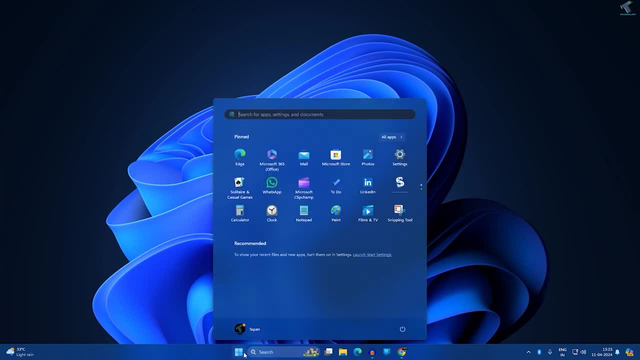 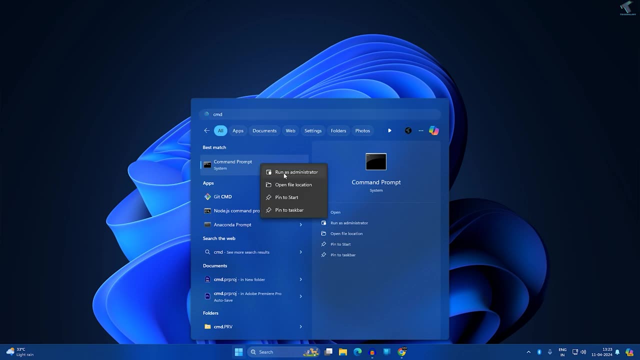 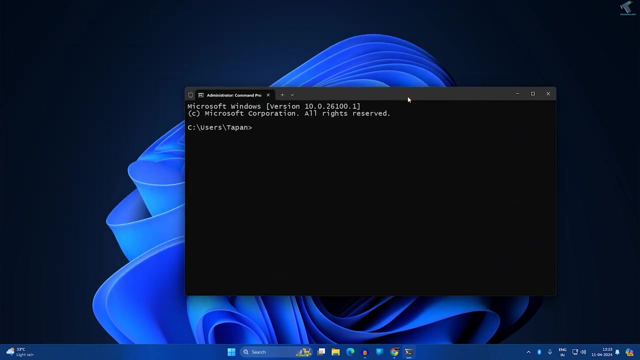 so after start your pc you just need to go to your start or search window, type over here: cmd. now open command prompt as an administrator. so right click and click on run as administrator and after open command prompt you just need to type one command which i'll give you on my video description. 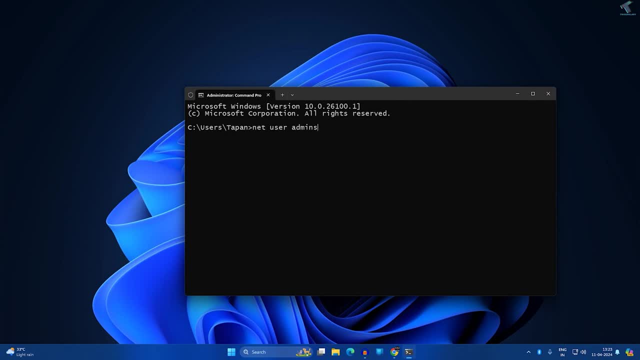 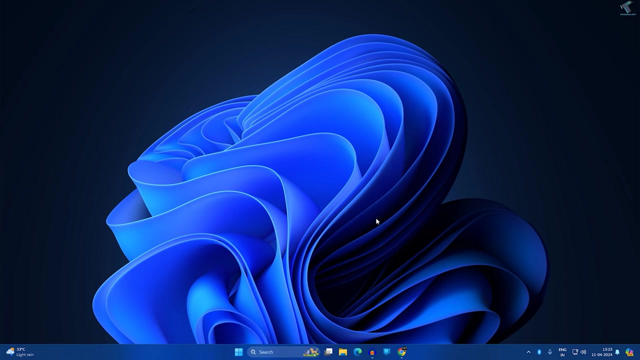 so the command is called net user administrator space slash active. then colon relate yes. after that press enter from your keyboard like command. so, as you can see, showing command completed successfully now what you have to do? you just need to close this window. also, you can use l user command to active your as administrative account. for that you just need: 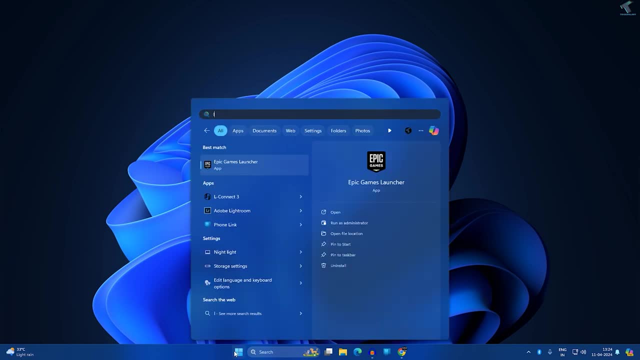 to go to your start or search window and type l? u, s, r, m, g, r, dot m s c. so i will give you this command also to my credits kitchen. after that type l user command, use your add to start or search window and type lusr, mgrmsc. so i will give you this command also to my view description. after thatj use PDF seeing how it would apply the back. 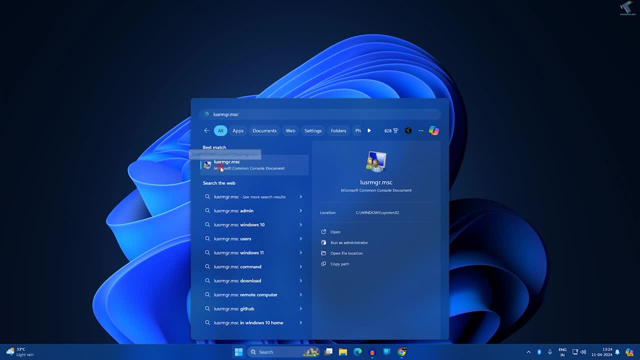 to my view description. after that type you are needed to go to start or search window and typeие disrmsc and type. I was waiting for an option after taking pictures, reading it will also give. after that, press enter or click on this app. after that you just need to. you will. 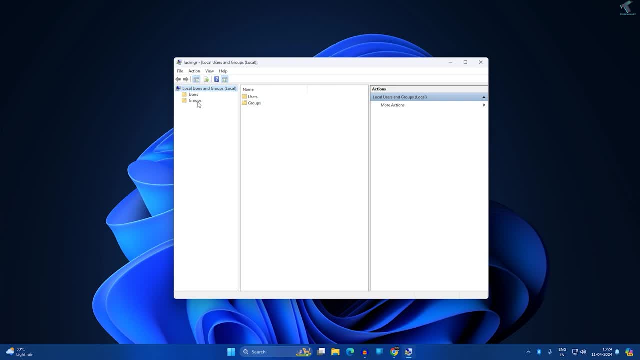 get two option, two folder, which is user and groups. so click on groups and here you will get. under groups you will get administrators, so double click on it and here you just need to click on add. so if you don't know your user account once username, then don't worry, just go to users and here you will get all your. 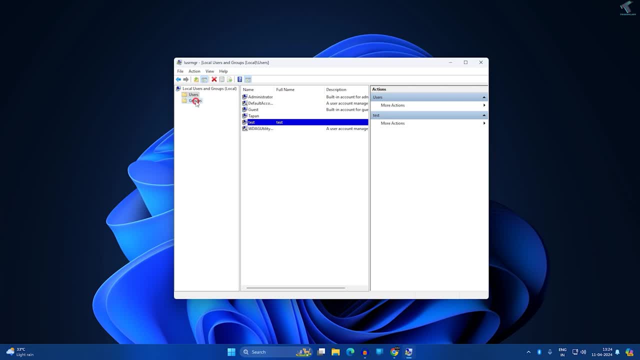 users. so I will do for my test account. so I'll go to groups and double click on it, then add, then here I just need to put my username, which is test, and click on check names. after that click on ok, then apply, then ok and try to uninstall your.